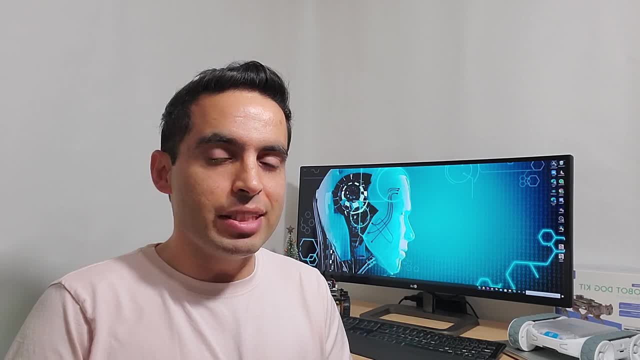 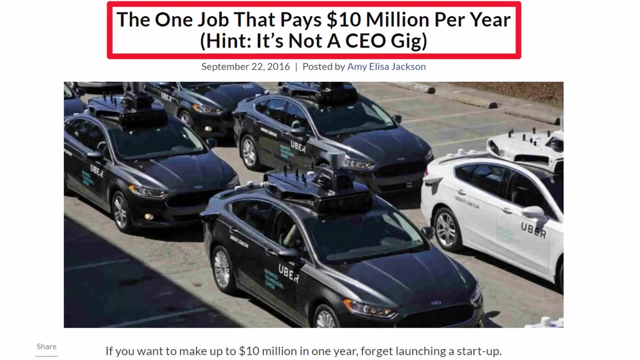 also known as self-driving cars. Tech giants are investing billions of dollars in R&D and startup acquisitions. There is a fight like hell for self-driving car engineers due to huge shortage of talent. Top robotics engineers in this field are paid as high as $10 million a year, according. 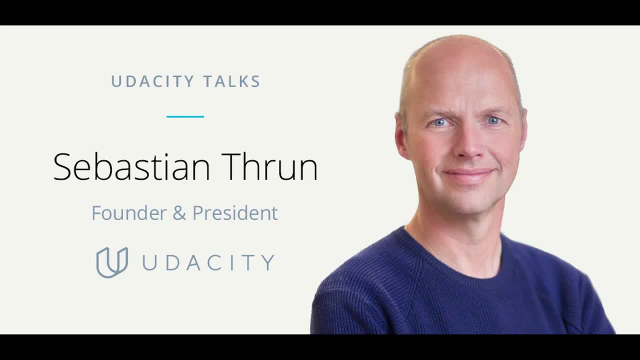 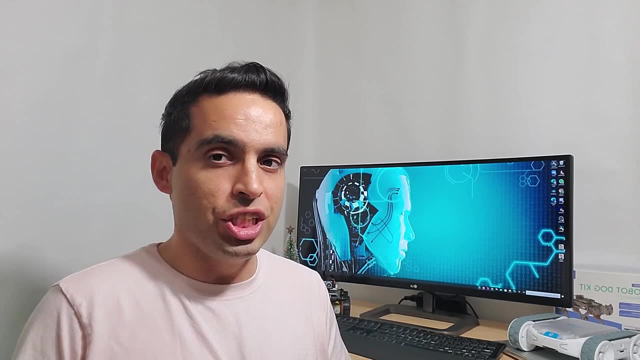 to Sebastian Throne, who is known as the father of robot cars. Money aside, these robotics engineers could potentially save hundreds of thousands of lives each year, which is more than enough to save hundreds of thousands of lives each year, which is more than enough to save hundreds of. 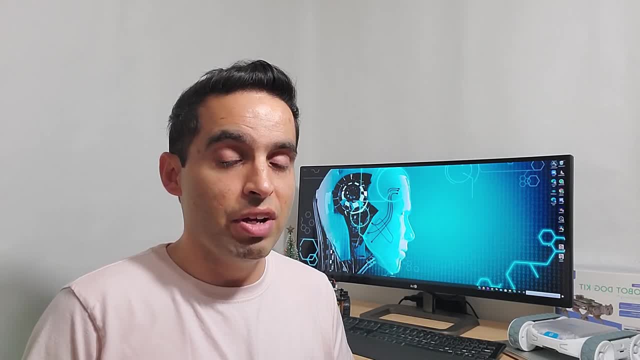 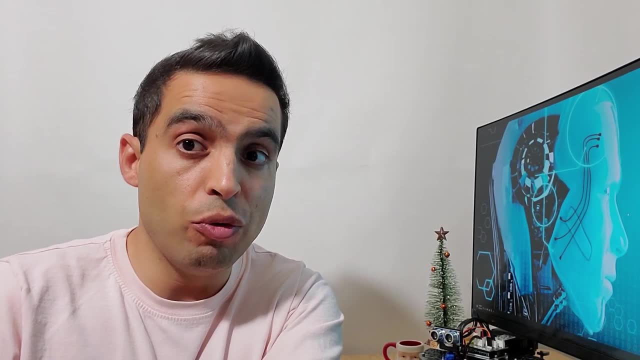 thousands of lives each year, which is more than enough to save hundreds of thousands of lives each year than a cure to a deadly cancer could potentially save. What's more rewarding than that? right? Alright now, how can you become a self-driving car engineer, and what are the required skills? 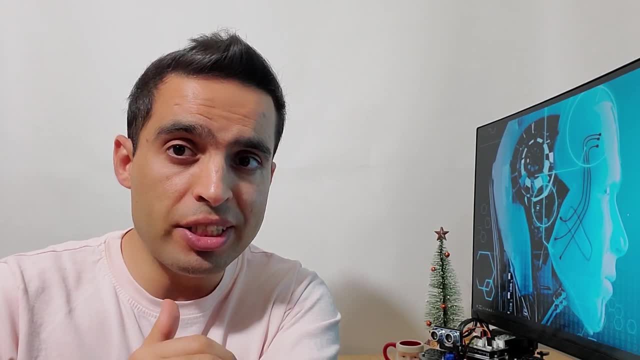 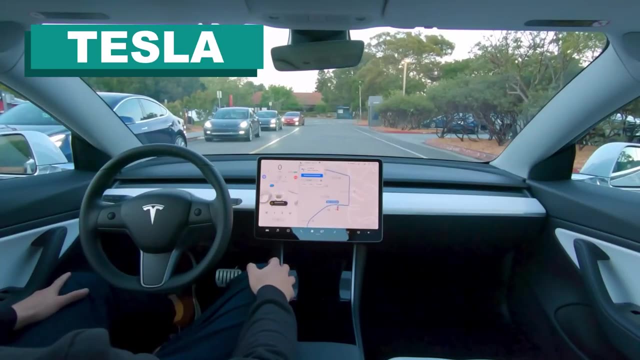 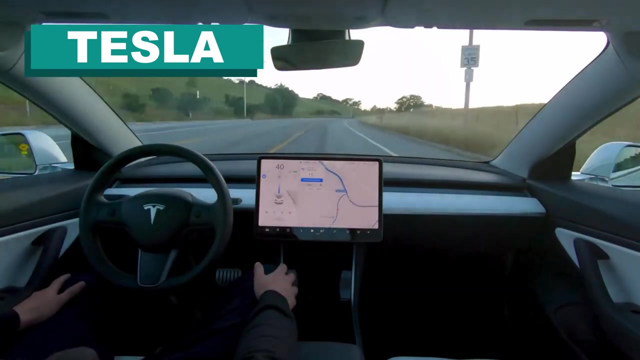 We will get to that, but first, who are these giant tech companies that are hiring self-driving car engineers? Well, the leading company is Tesla. While Tesla is the head of the game with their own AI chip and more than 3 billion miles worth of data, the following companies are playing catch up: The 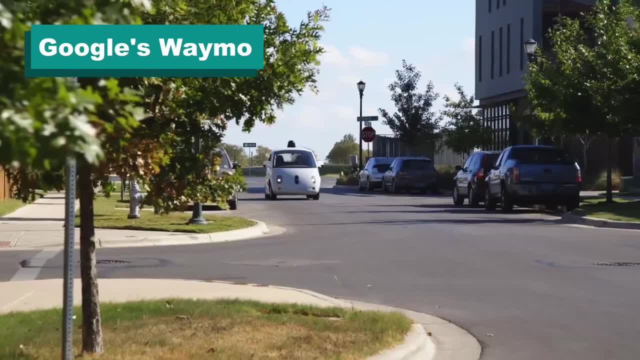 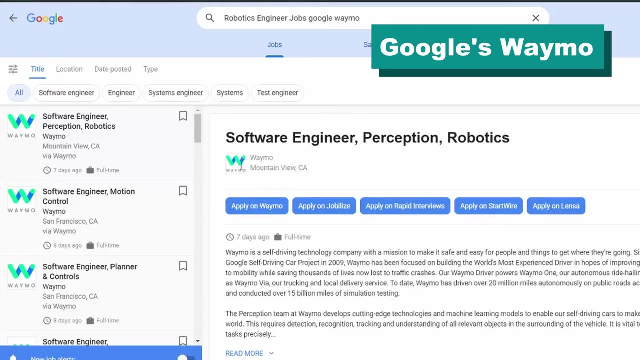 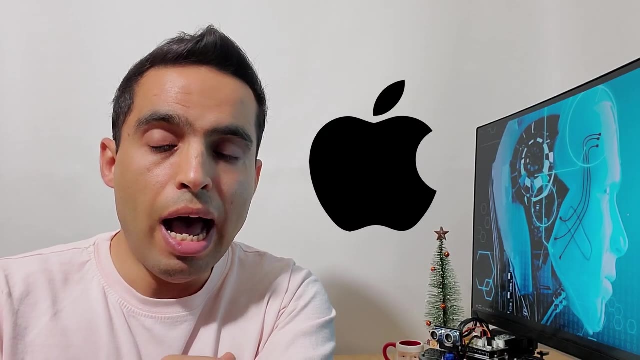 first company is Google. Google's Waymo is developing autonomous driving technologies, including ride-hailing service, trucking and local delivery services. Waymo has a ton of open positions for robotic software and hardware engineers. The second company is Apple. Apple is developing autonomous systems, including a self-driving car. 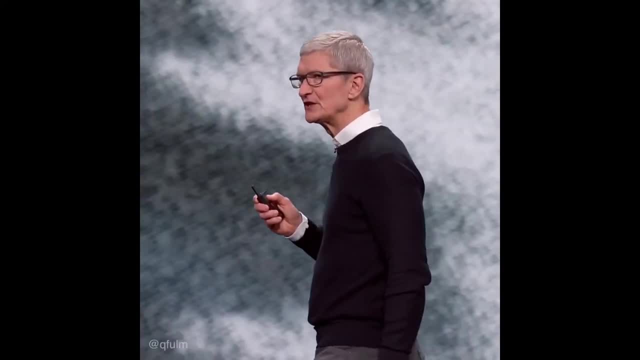 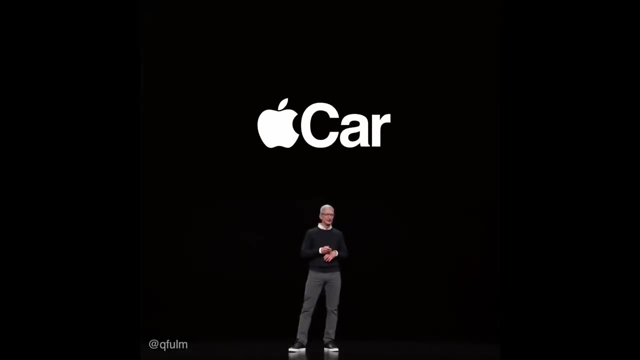 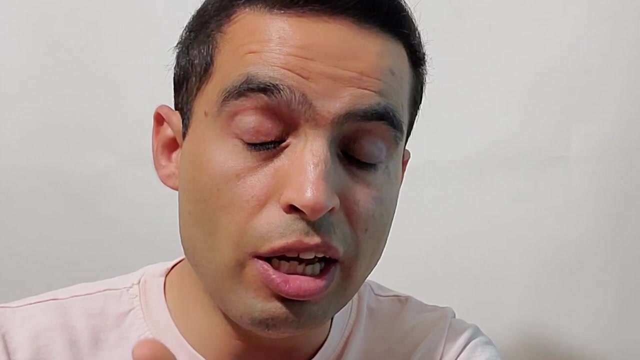 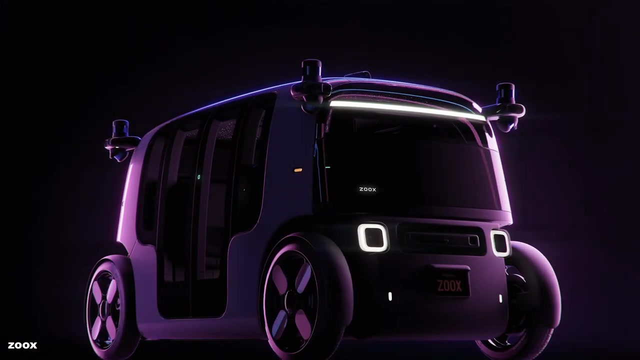 called Apple Car And we saw an opportunity to transform another fundamental method of transit. The third company is Amazon. What does this new software call? again, The third company is Amazon. Amazon's Zeusk just recently rebuffed a prototype of its robot taxi called I don't know. 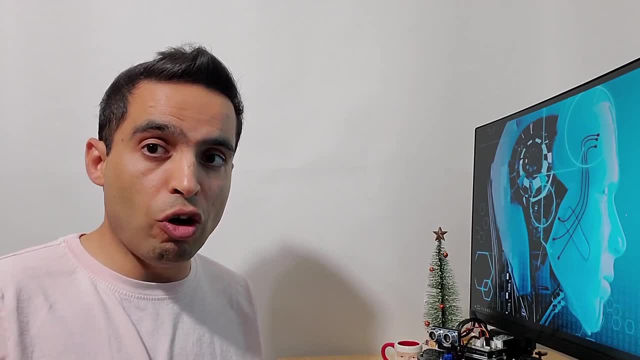 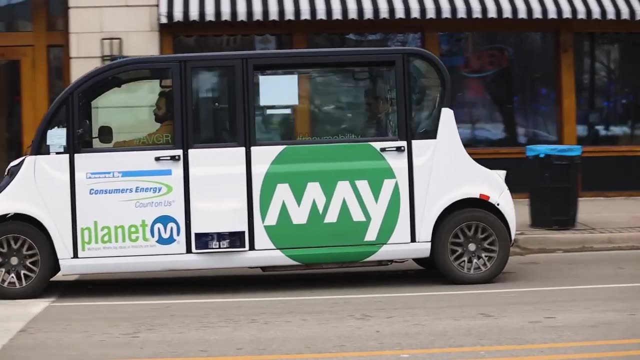 And Amazon's Zeusk also has a ton of open positions for robot software engineers: Amazon's Zeusk, which will be planning a full scale robot taxi in system technology. Apart from these high-tech companies, Uber and Lyft: both are working on robot taxis. 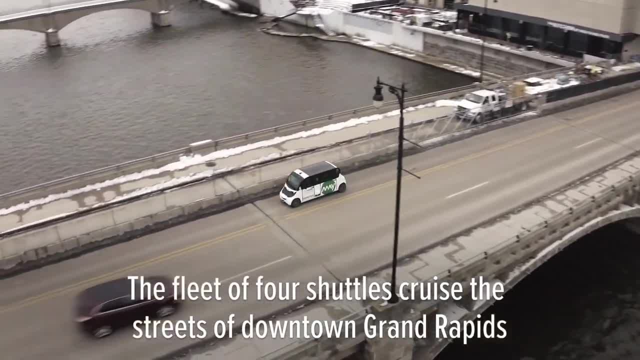 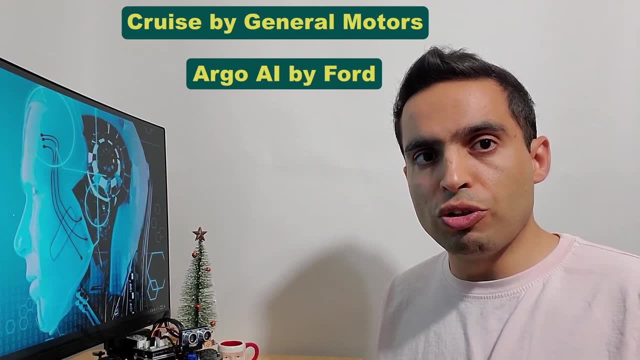 and almost all automakers are developing a robot car. Just to name some, we've got Cruise by General Motors, Argo, AI by Ford, and also, from the startup world, you've got TuSimple, Torque, Aurora and many more. 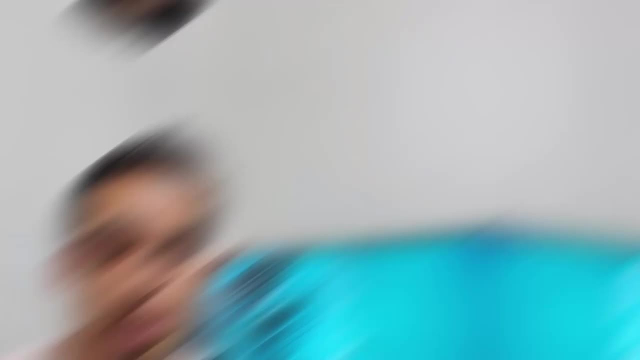 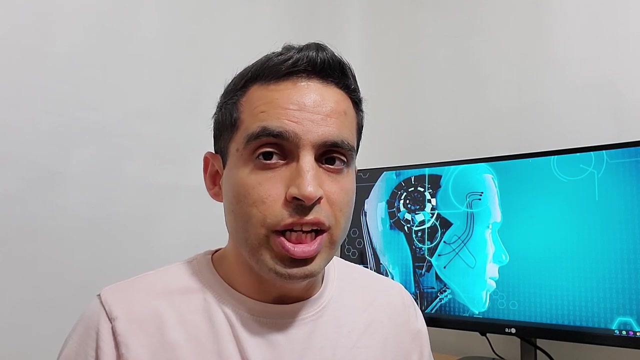 Just please refer to the description box for an updated list. But, Sina, I'm not living in the United States. What about other countries? Well, autonomous vehicles is a global trend and, honestly, it's more of a race between different countries. 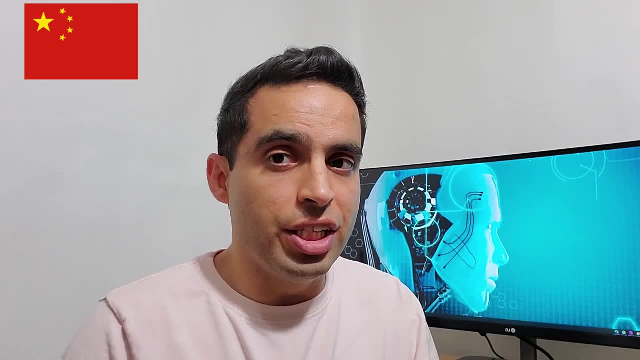 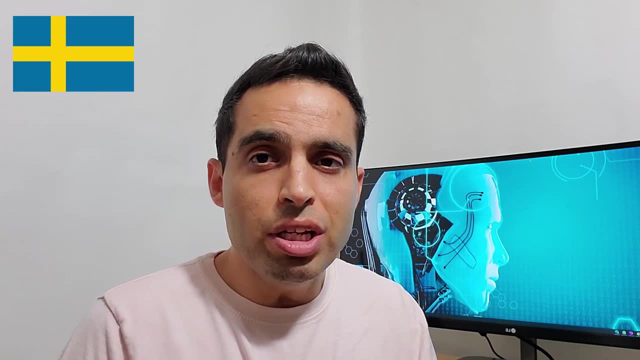 The most serious competitor to the United States is China. In China, you've got Pony AI, Alibaba, Baidu, Didi, and the list goes on and on. In Sweden, Volvo is developing autonomous trucks, in addition to startups like Autoliv and Einride. 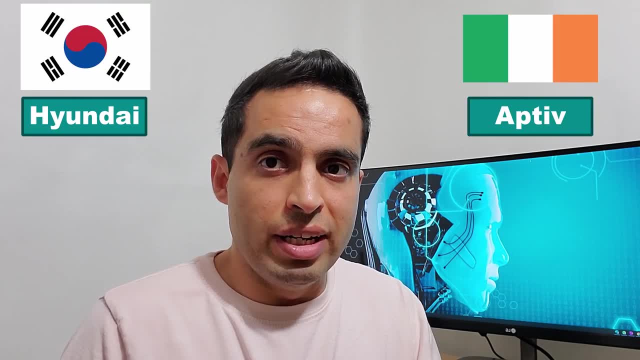 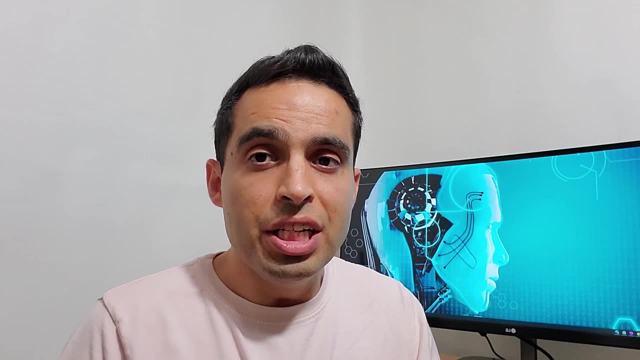 Also, we've got Hyundai in South Korea and Aptiv in Australia, In Ireland, In Germany, almost all automakers are developing self-driving cars, including Audi, Mercedes and BMW. In India you've got Nvidia, Bosch, Mercedes. 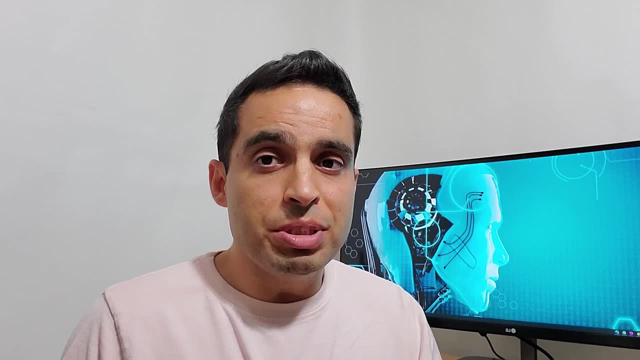 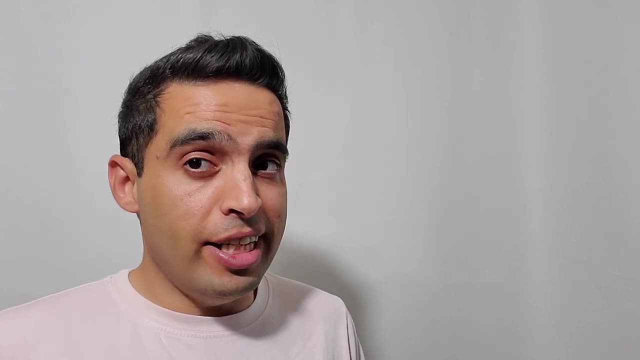 Flux Auto and a couple of others. There are companies and startups in France, Israel, Canada, Japan and Russia. Okay, now do you need to go to MIT, Stanford or other universities to become a self-driving car engineer? 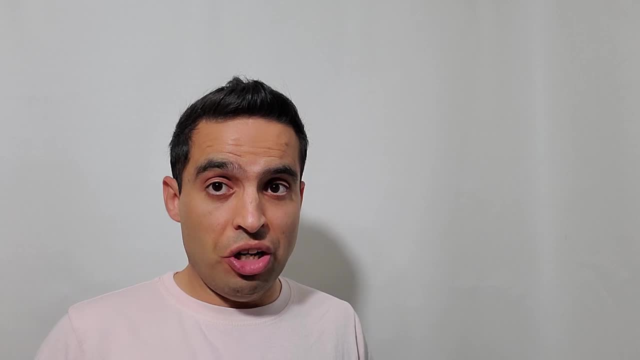 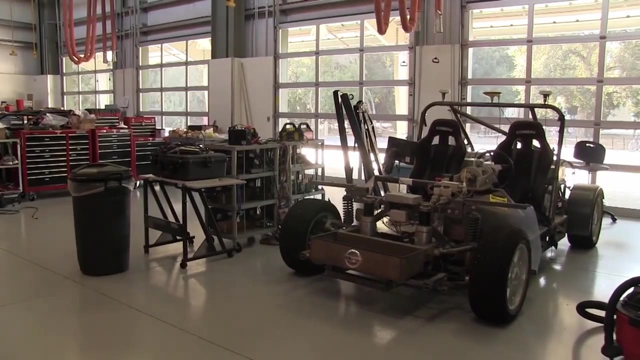 Absolutely not. As a matter of fact, Udacity, which is an online agency, an educational platform, has trained more self-driving car engineers than any institutions in the world. If we can build a safer car, we would save a lot of lives. 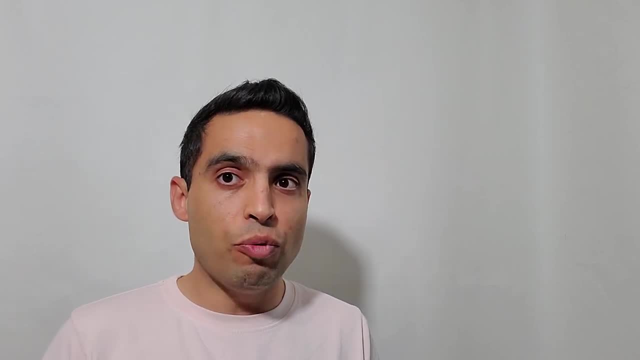 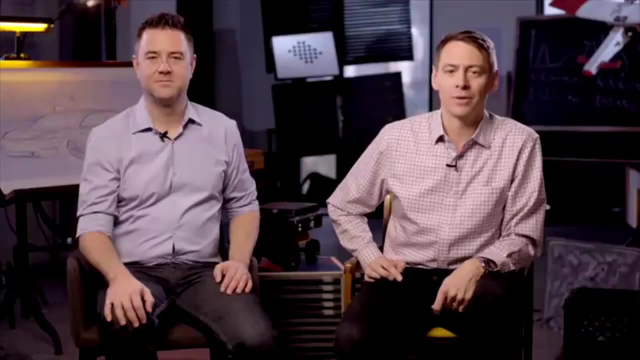 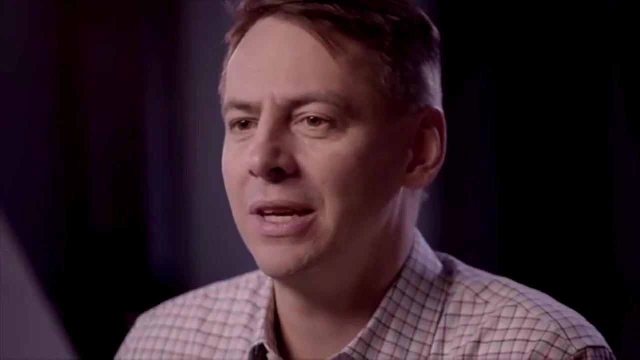 Udacity offers two nanodegree programs: one for beginners and one for people with background in programming and math. Coursera also offers a self-driving car specialization. Whether you're coming from academia or industry, these courses will provide you with the foundational knowledge and practical skills. 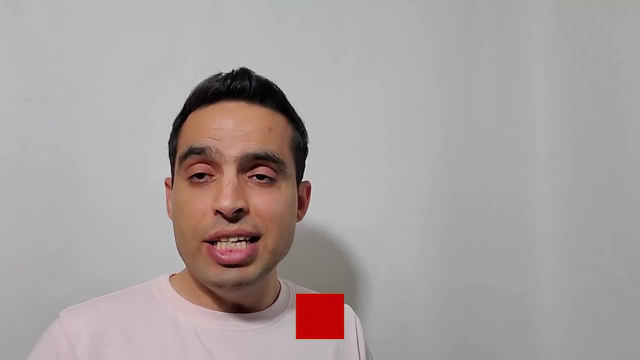 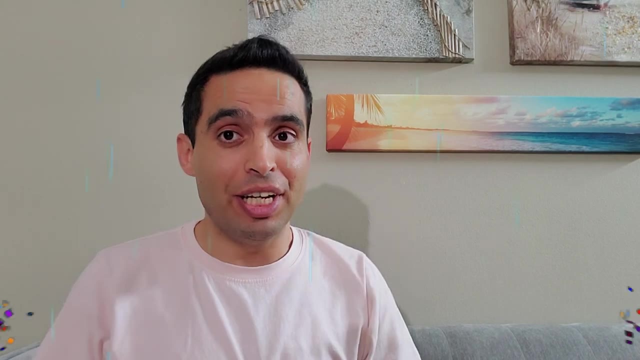 you need to help build a new future with self-driving cars. Please refer to the description box for links to all of these programs. All right now is the time for a surprise giveaway If you happen to enroll in any of these programs through my referral links. 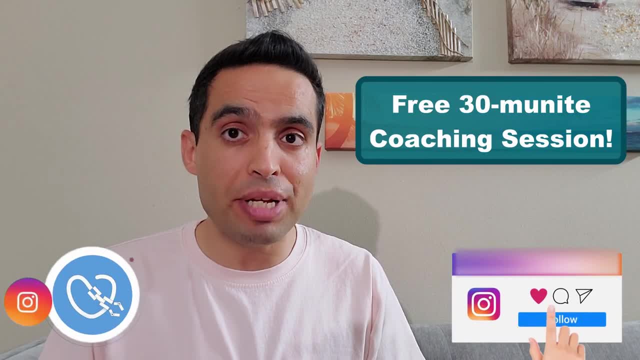 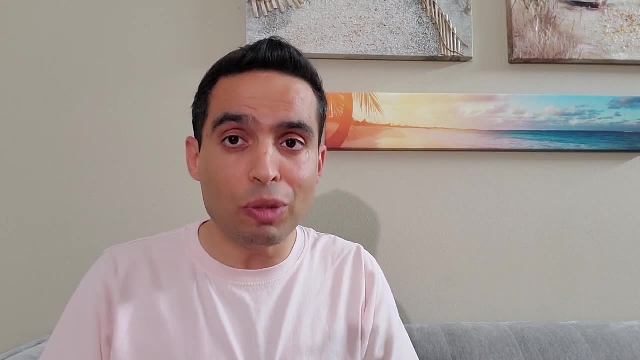 please direct message me on Instagram and I'll give you a free 30-minute coaching session, which is worth $50.. Now, if you don't wanna pay for any of these online programs, but you still wanna become a self-driving car engineer? 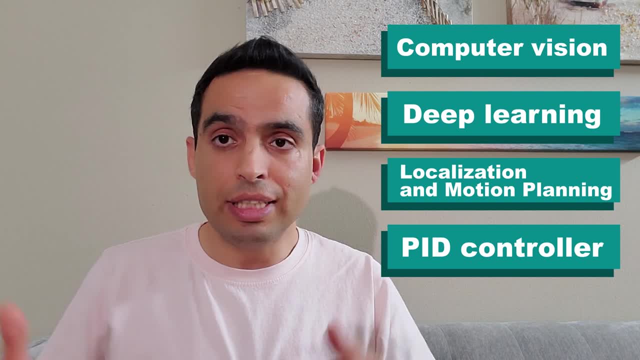 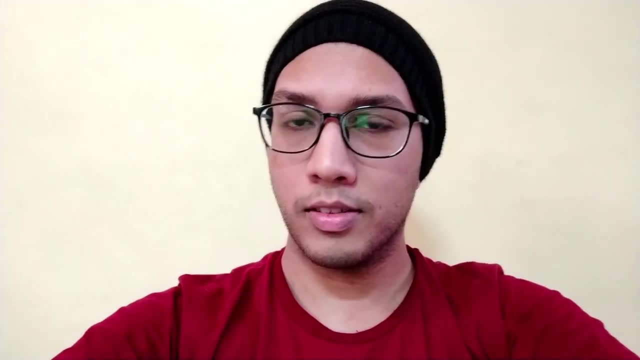 here are the skills you need to learn: Computer vision, deep learning, localization and motion planning and PID controller. But, Sina, these are software skills. How about hardware skills? That's right, my friend, Robotics. car companies hire a lot more. 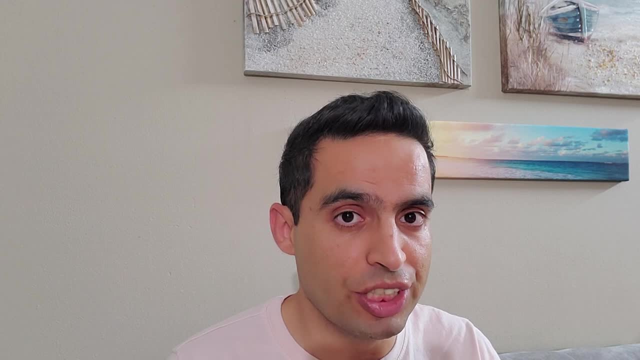 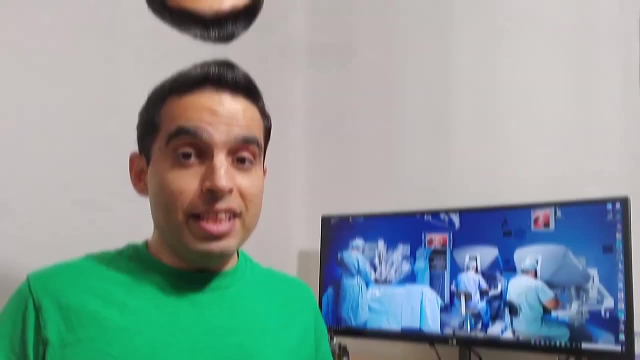 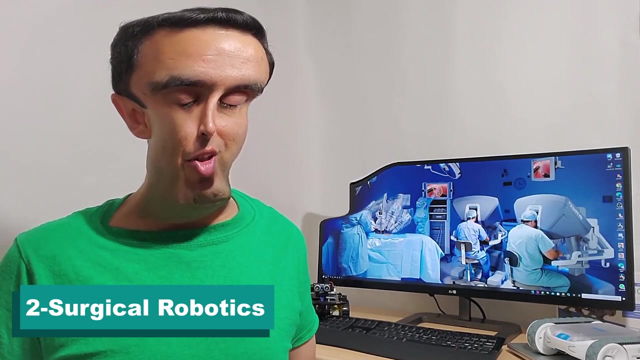 robotics software engineers than robotics hardware engineers, But why? We'll talk about that in a separate video, But for now, please subscribe and stay tuned. All right, the second hottest field in robotics, and my favorite, is surgical robotics. I'm a surgical robotics engineer after all, right. 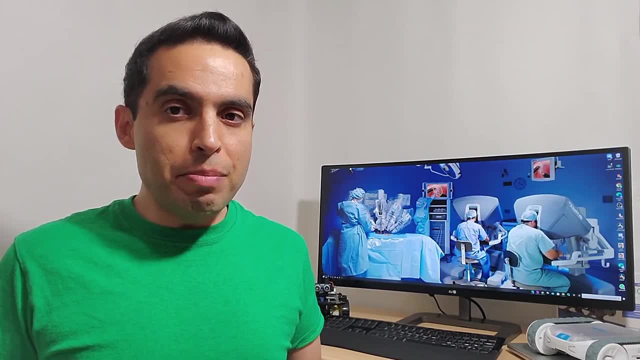 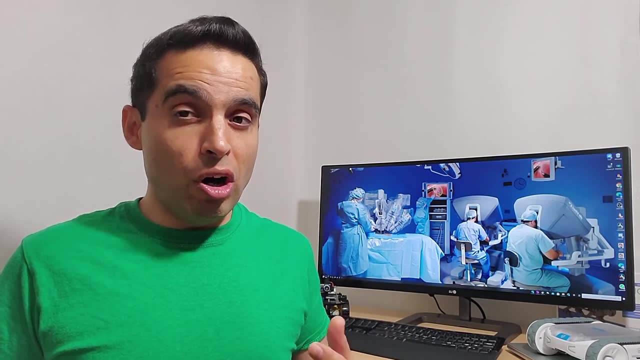 Now surgical robotics is growing like crazy. Almost every month a new surgical robotics startup pops up out of nowhere. All major medical device companies either already have a surgical robot in the market or are developing one. Don't believe me? Look at this image. 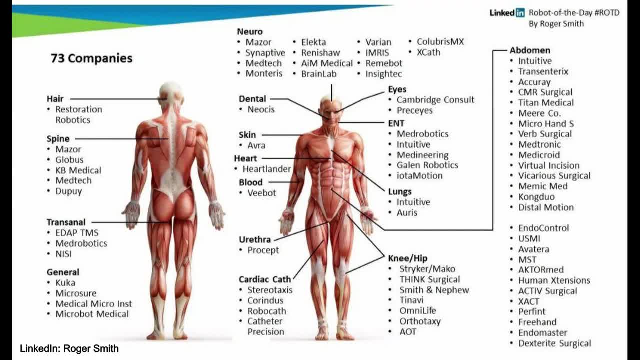 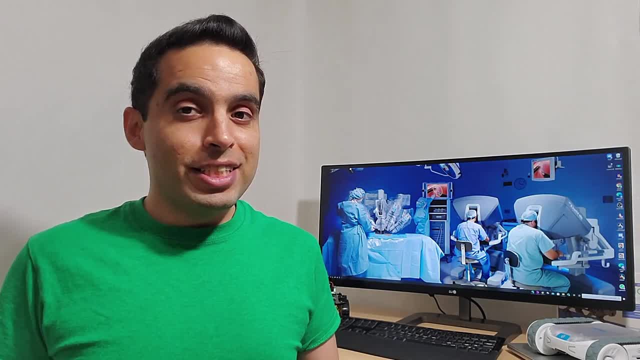 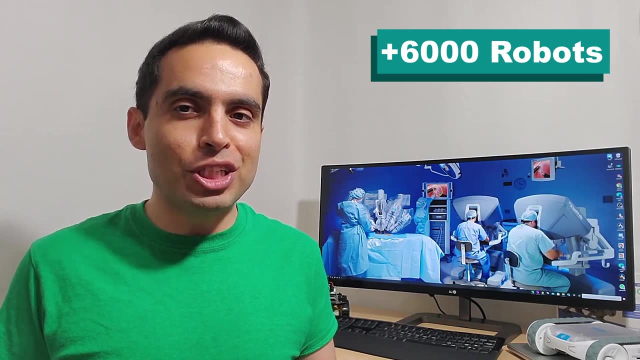 Soon there will be a robot for almost any organ or joint of the human body. Unlike autonomous vehicle companies who are still testing robot cars, surgical robotics companies have already installed more than 6,000 robots, which have been used in millions of surgeries so far. 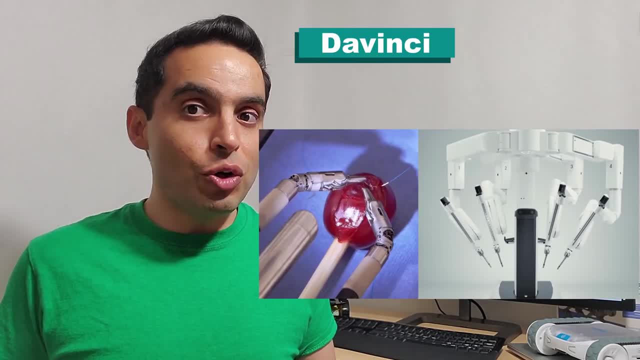 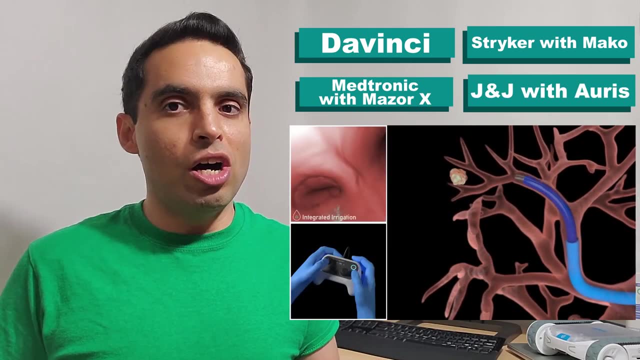 Key players are Intuitive Surgical with DaVinci, Robot Striker with Mako, Metronic with Mazora X, J&J with Oris, and the list goes on and on. So these surgical robotics companies are all competing for a limited pool of talent in the field. 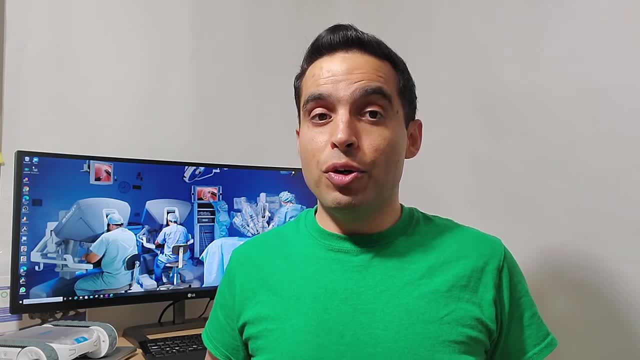 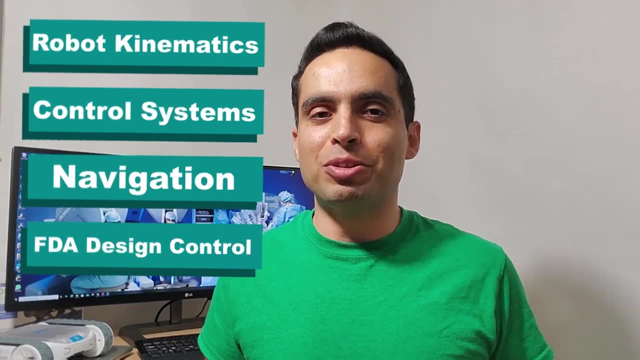 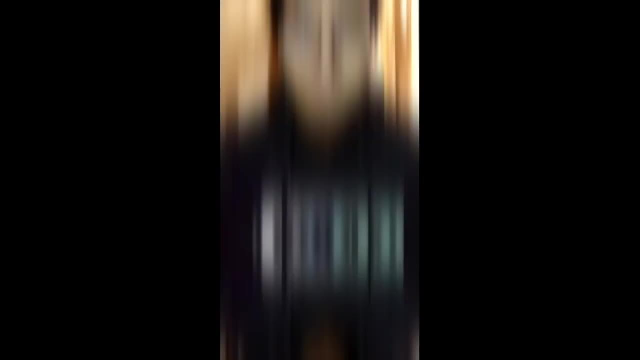 So if you pick up the following skills, you'll be in high demand: Robot kinematics, control systems navigation and FDA design control. Hey Sina, You're a surgical robotic engineer. What's it like to be a surgical robotic engineer? 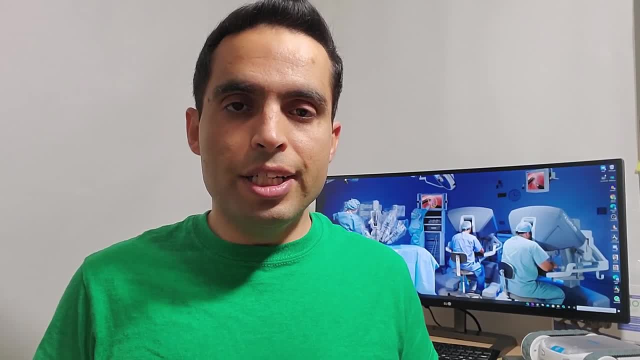 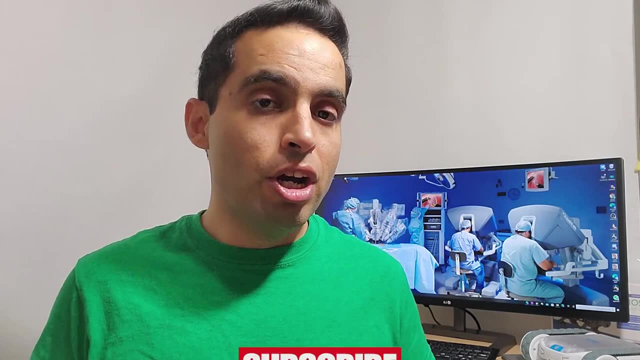 Well, the only thing I can tell you is that I love what I do, especially the feeling that my work makes a positive impact on quality of life of hundreds of thousands of patients each year. More on that in a future video, and another reason for you to subscribe. 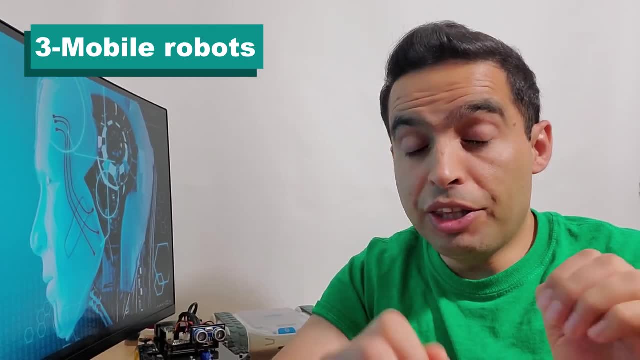 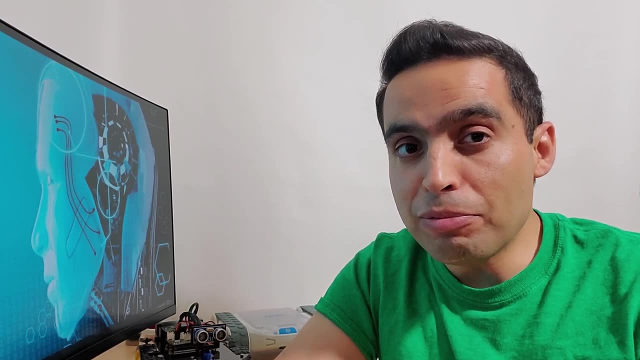 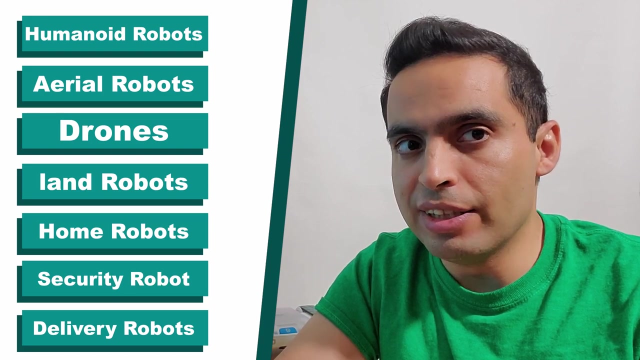 All right. The third field is mobile robotics. Autonomous mobile robotics is another field in robotics that is growing fast. Mobile robotics has its own subfields. that includes humanoid robots, aerial robots or drones, land and home robots and security and delivery robots. Well, with the autonomous vehicles becoming mainstream, there will be a growing 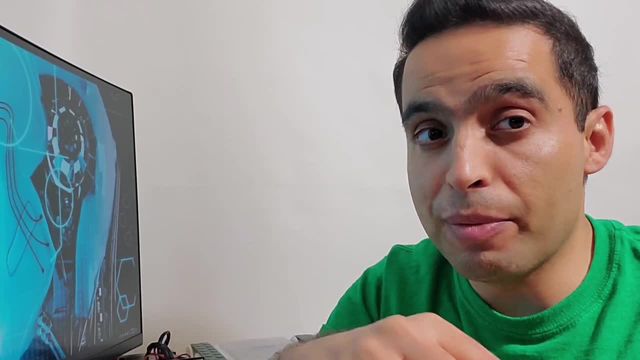 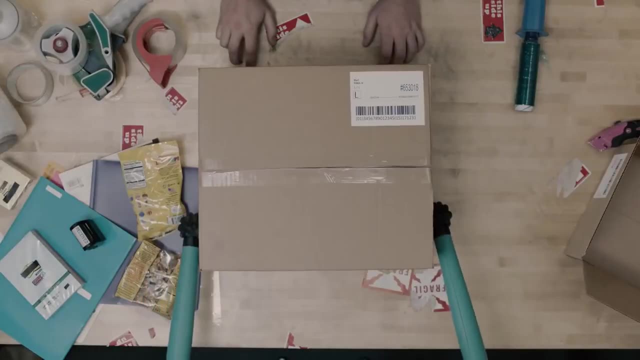 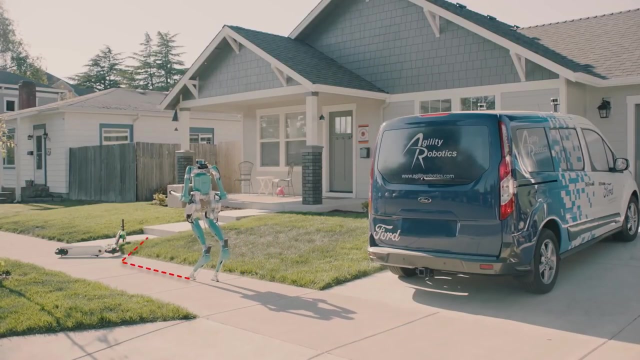 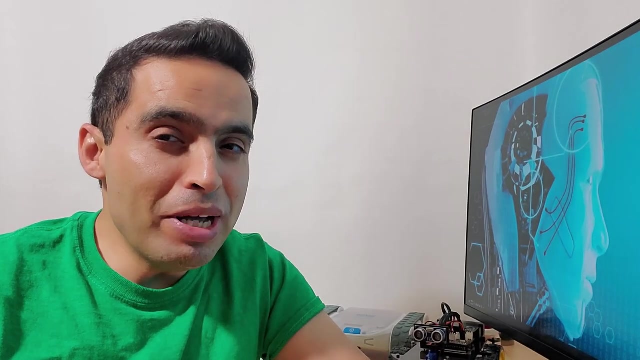 need for humanoid robots that can take your package from the autonomous van and deliver it to your door. You think this is too futuristic? You're wrong. This is exactly what Ford and Agility Robotics are working on right now. A dream place for many robotics engineers is NASA. 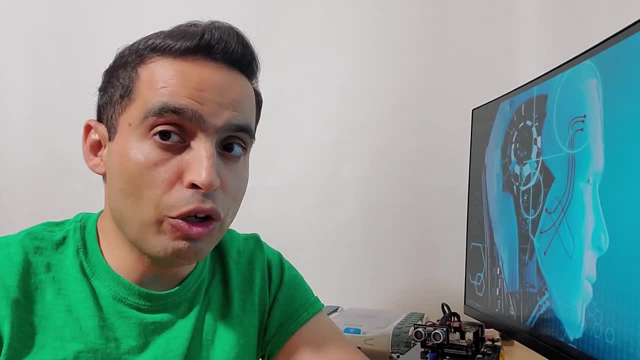 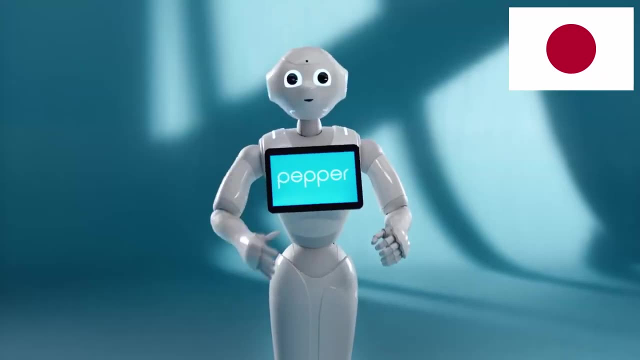 NASA, JPL hires robotics engineers for development of the rover and Robonaut. Japan is probably the leading country when it comes to humanoid robots, with Pepper by SoftBank, Asimo by Honda and Nautilus. Japan is probably the leading country when it comes to humanoid robots, with 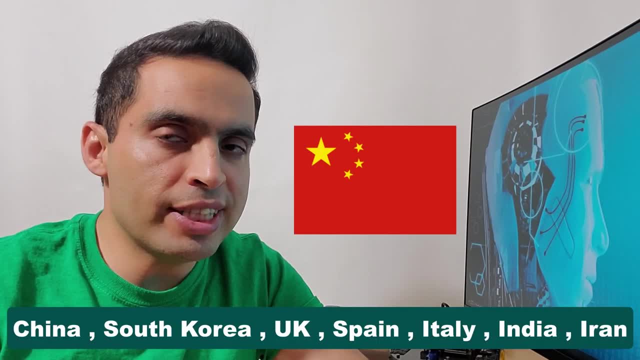 Pepper by SoftBank, Asimo by Honda and Nautilus. Japan is probably the leading country when it comes to humanoid robots, with Pepper by SoftBank, Asimo by Honda and THR3 by Toyota. There are companies in China, South Korea, UK, Spain, Italy, India and Iran who are developing humanoid robots. 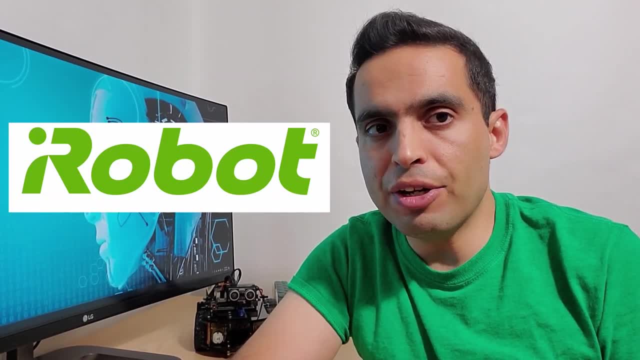 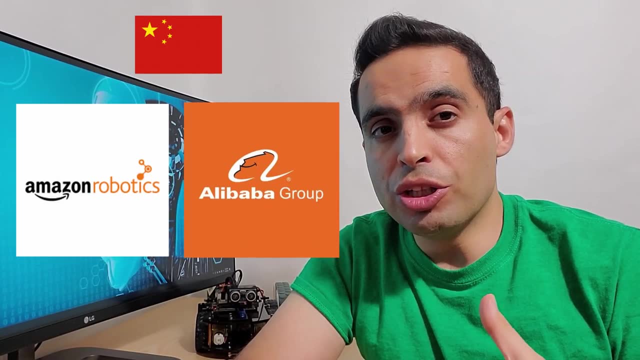 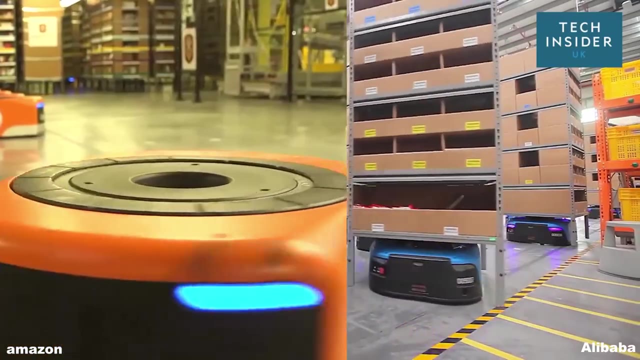 When it comes to home robots. iRobot is the leader with the Roomba vacuum robot and Terra, the robot mover. Amazon Robotics and Alibaba in China are the two giant companies who are making warehouse robots and delivery drones. They both are big recruiters of robotics engineers. I know what your 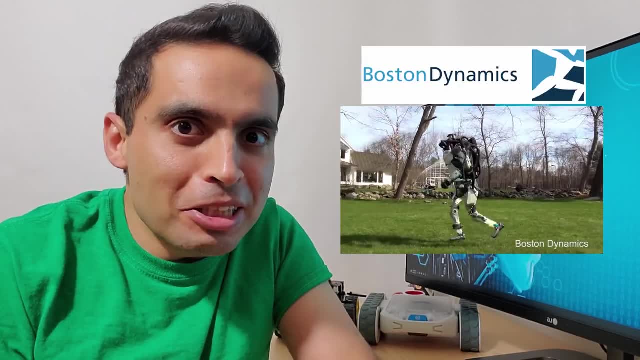 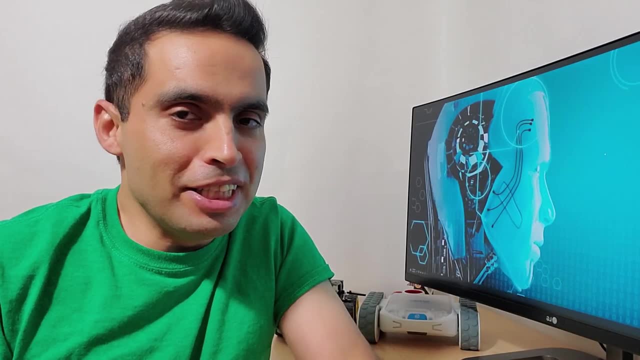 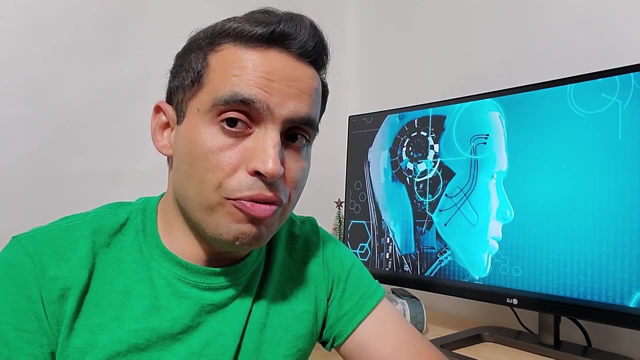 thoughts are dying to ask now, Sina, you forgot Boston Dynamics. Of course I did. Boston Dynamics and Hanson Robotics, the company who makes SOFIA, do not need any introduction, right. Okay now how to become a mobile robot engineer? Well, Udacity offers a great comprehensive nano. 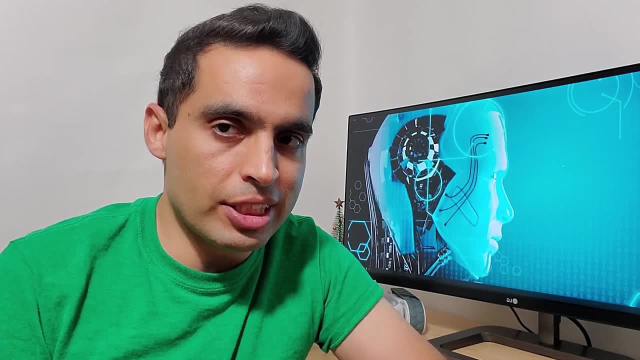 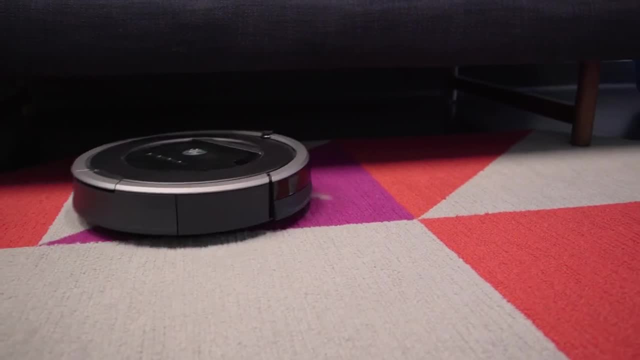 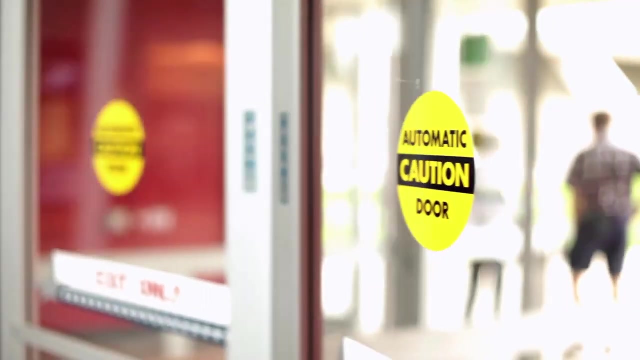 degree program that teaches you all the essential skills for mobile robot. We have robotics in space, in toys, in your home. If you think about the definition of robotics, which is sensing, thinking, making a decision and then taking an action, so many things in our world are using robotic technology. 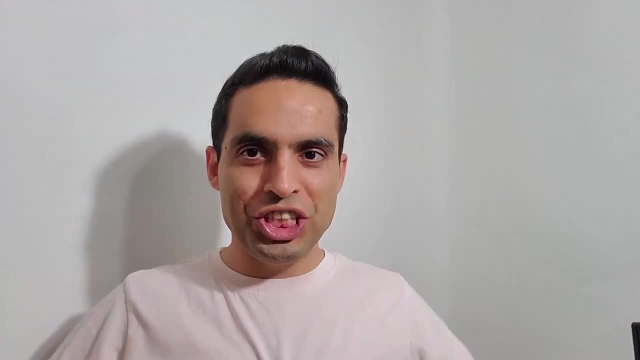 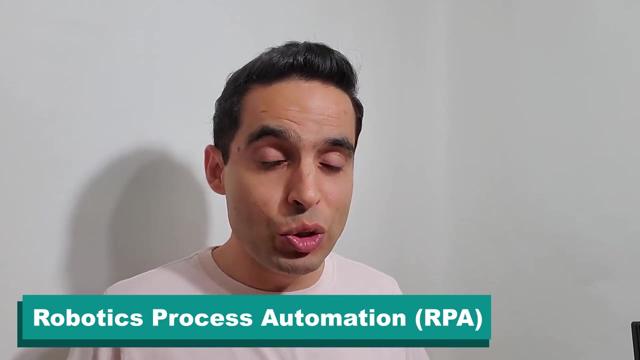 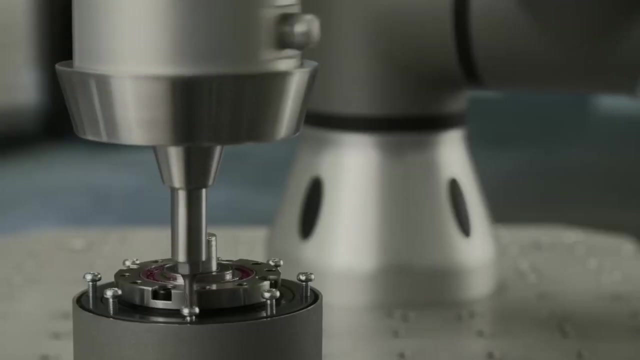 The link is in the description box. All right. what else is hot in robotics? Robotics process automation is probably the fastest growing field in robotics. There exist more than 3 million industrial robots and collaborative robots, also known as cobot Robots, around the globe, automating almost everything from making cars and airplanes. 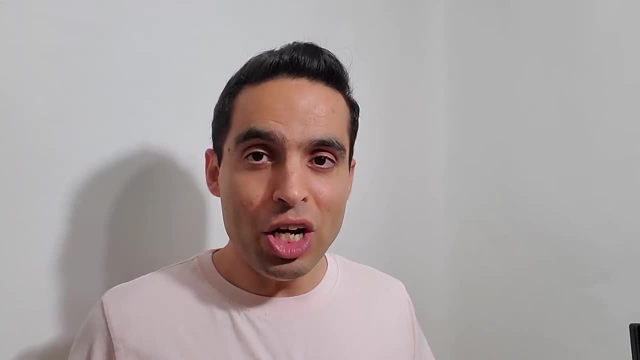 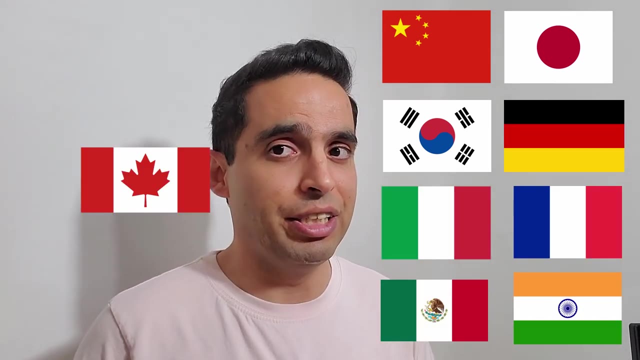 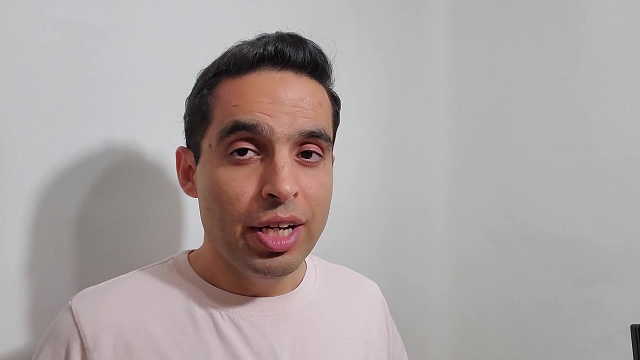 to even cooking burgers. Robotics process automation is hot in China, Japan, South Korea, Germany, Italy, France, Mexico, India and Canada. See the description box for a list of key players in this field. Okay, now, what's in it for you? The benefits for you is twofold. First, industrial robot manufacturers need robotics engineers to design and build more advanced and less expensive industrial robots each year. Second, the companies who use cobots, including automakers such as Tesla, need robotics engineers to program these robots to automate manufacturing processes. 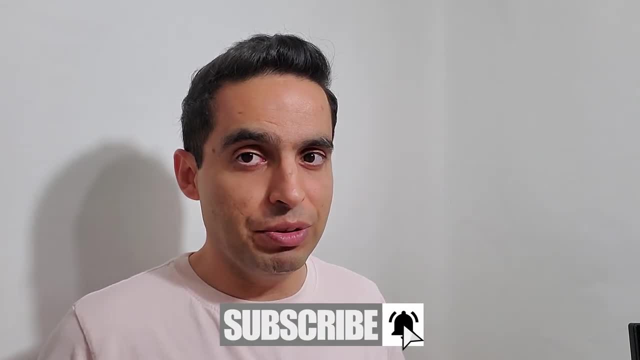 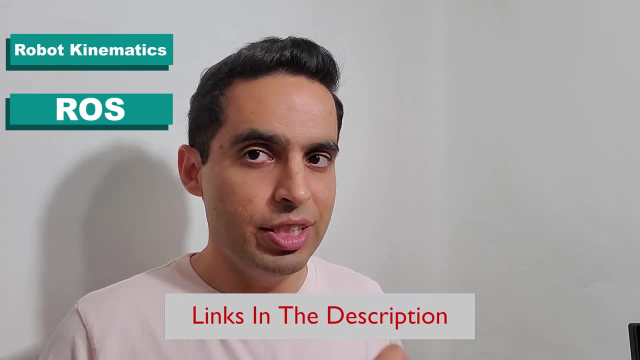 Now what are the skills you need to pick up for this field? The key skills are robot kinematics and ROS. Refer to the description box for resources to learn these skills. 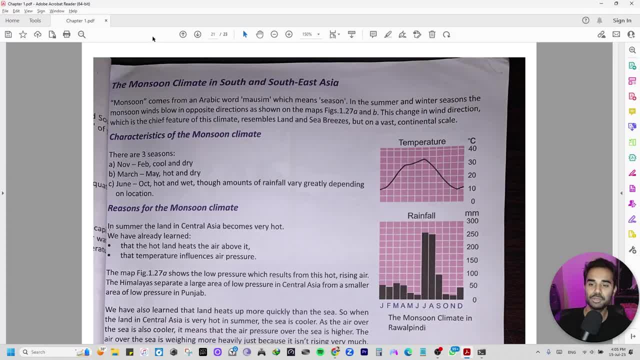 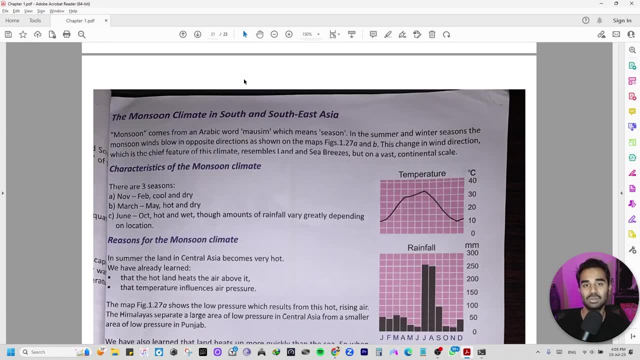 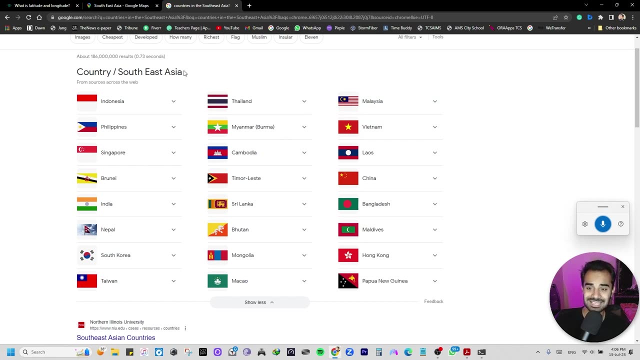 Now, guys, we're going to understand the monsoon climate in South and Southeast Asia. Okay, Now you need to understand what do we call South and Southeast Asia? So just bear with me, Let me show you on the map. So, guys, now, first, these are the countries which are part of the Southeast Asian. 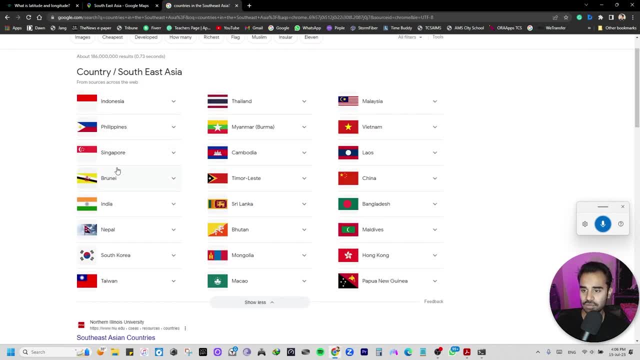 region on the planet Earth. Okay, So we have Indonesia, Philippine, Singapore, Brunei, India, Nepal, South Korea, Taiwan, Macau, Mongolia, Bhutan, Sri Lanka, Timor-Leste, Cambodia, Myanmar, Thailand, Malaysia, Vietnam, Laos, China, Bangladesh, Maldives, Hong Kong and Papua New Guinea. 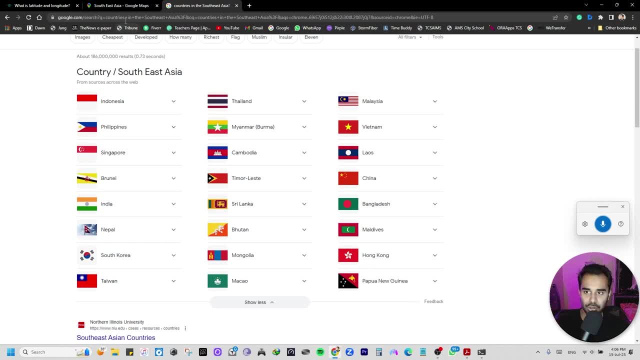 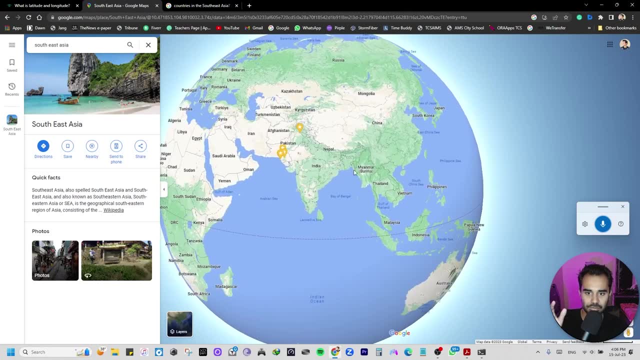 Right. So these are all the parts, part of the Southeast Asia, as per the Google, And actually this is a kind of you know entire world map of these countries of the Southeast Asia. So, okay, We're right now here in Pakistan And, for instance, we have India over here. 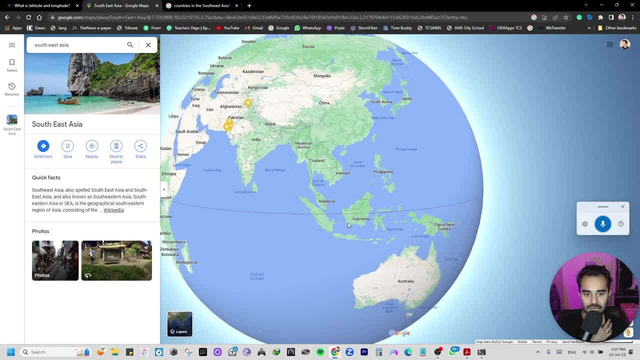 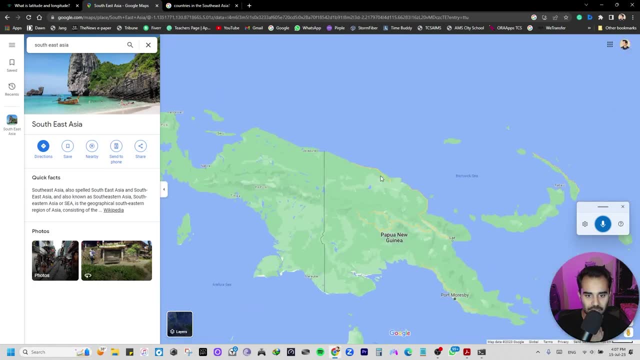 the Sri Lankas over here, the Burma, Thailand, Vietnam, Malaysia, Indonesia, Philippines is right here, And then we have the Papua New Guinea. Okay, This is Papua New Guinea over here. Right, This is Papua. This is.